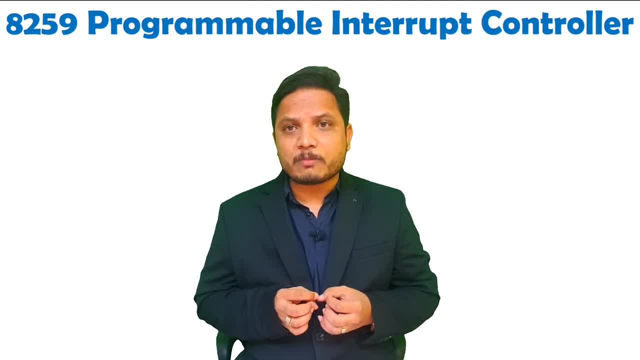 in that there were few interrupts that can be handled by those microprocessor, Like if you see 8085, in that there were only 5 hardware interrupt. Out of all those 5 hardware interrupt, only 3 interrupt that can be masked by 8085. But as if you interface 8259, programmable. 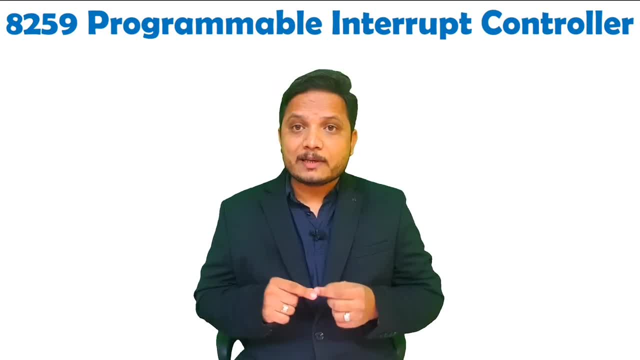 interrupt controller IC with microprocessor. in that case we can increase interrupt handling capacity. Here total 8 interrupts that can be handled by 8259.. And if you further want to increase capacity you can increase the capacity of the microprocessor. So if you increase the 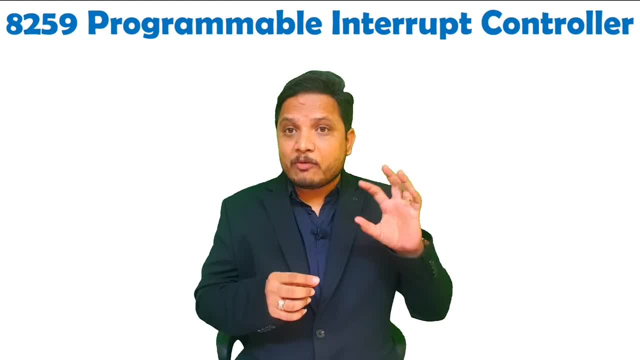 capacity of the microprocessor. you can increase the capacity of the microprocessor. So if you, then by having one 8259, we can have one master 8259.. Along with that we can interface 8- 8259 and we can increase interrupt handling capacity up to 64 interrupts. So here our agenda is to 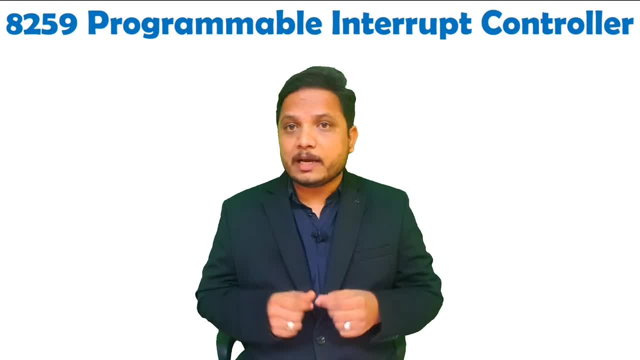 increase interrupt handling capacity, and that's why we use 8259.. Now, my dear students, what I'll do is I'll explain you features of 8259, its block diagram as well as its working, so that it will give you a clear idea about how 8259 functions. So let us see first how many features are there with. 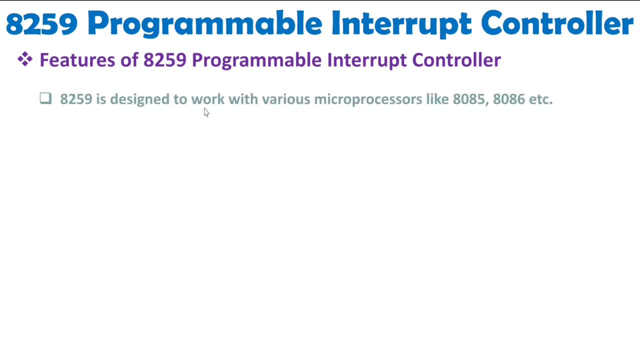 8259.. So, my dear students, with 8259, we have designed this IC to have working with various microprocessors like 8085, 8086, and it will increase capacity of interrupt Here. with single 8259 IC we can handle 8 interrupts and if you further want to increase capacity of interrupt, 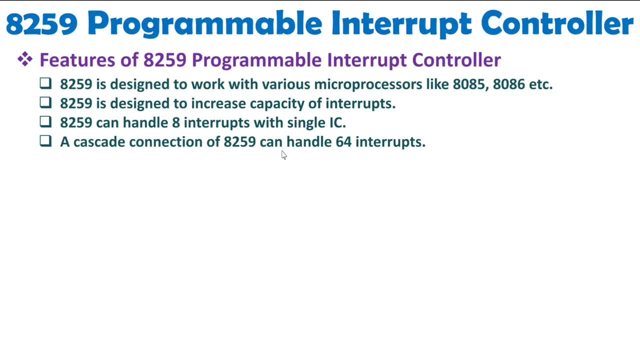 then you can have it up to 64 interrupt in which one master 8259 can work with 8 slave 8259 and it will increase capacity up to 64,. right 8 into 8 means total 64 interrupts can be handled over here. 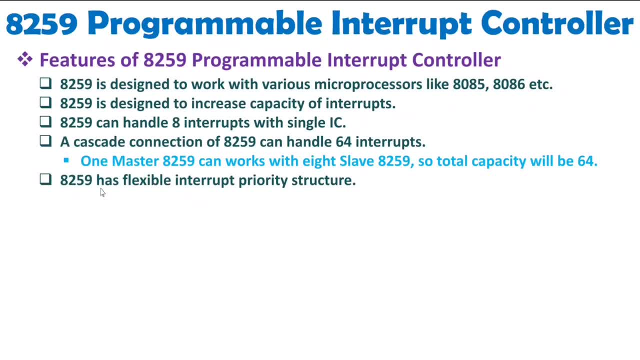 Here there are many features, which is there with 8259.. Here you'll be having flexible interrupt priority structure. We can mask all the interrupts and here all the vector address that can be programmed at the side of 8259, right, So all the vector. 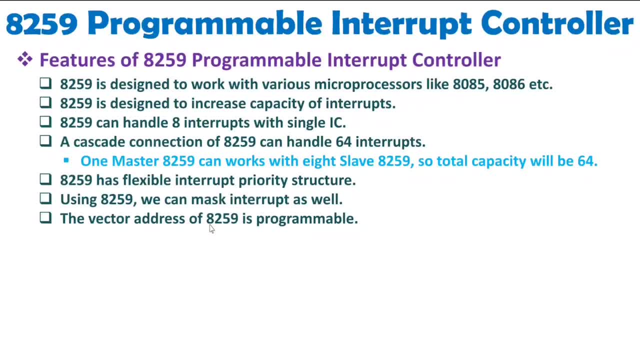 address are programmable. Why? The reason is: with 8259, we'll be generating call and with call instruction we can provide any address right, So vector address is programmable, While with 8085, we were been having RST instructions, where vector address of RST instructions were fixed. 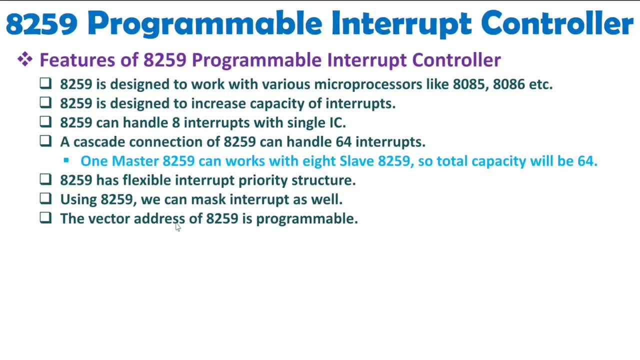 But by using call we can provide any address. So we can provide any address. So we can provide any call instruction. We can have vector address programmable by using 8259.. Here status of interrupt can be observed by microprocessor and that we can have it by having pending status. 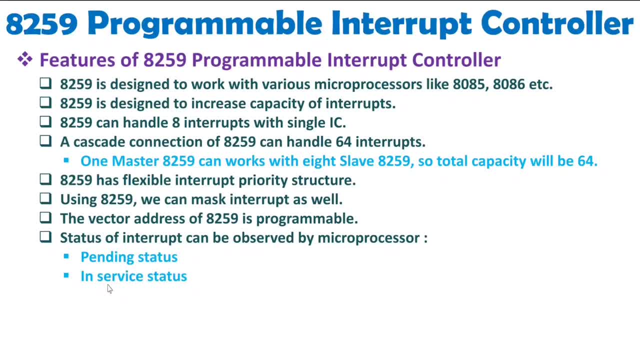 as well as we can see which interrupt is in service right now, as well as we can mask the interrupts. So how to do all those things? Let us try to understand that step by step. So first of all, I'll be going to explain you a basic architecture. So in that, 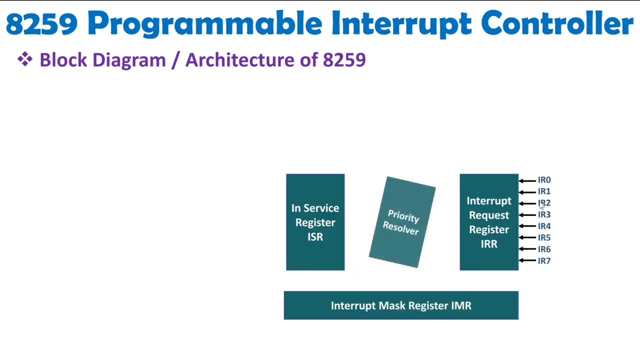 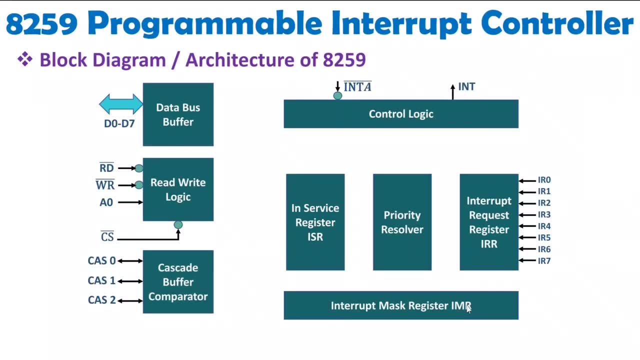 with IIR register we can take 8 interrupts and in service register will show you which interrupt is there in service interrupt mask register. that will gives you idea about which interrupts are masked. right now Control logic is connected with INT and INTA bar, This INT terminal that is connected. 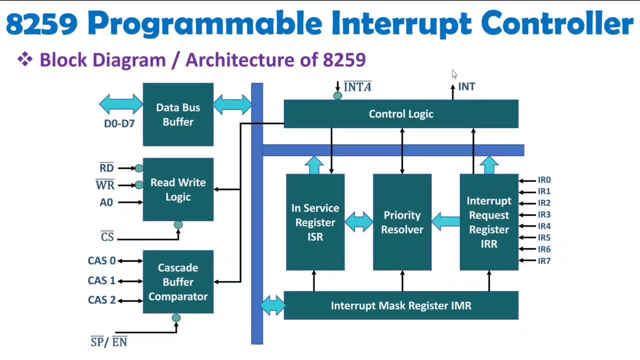 with microprocessors. INTR terminal and acknowledgement terminal of microprocessor is connected over here at INTA. bar Cascade buffer is connected with system bus D0 to D7.. Read and write control logic is available over here along with chip select and this cascade buffer comparator that is. 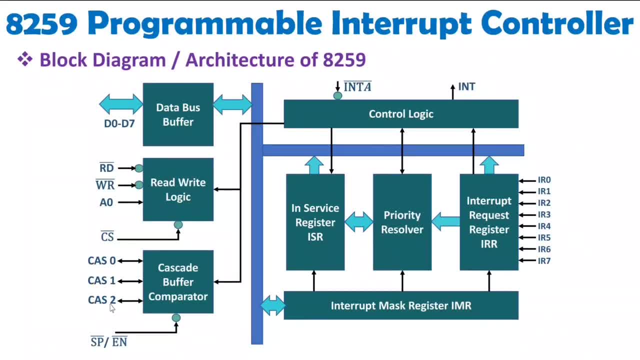 having CS0, CS1 and CS2 to increase capacity of interrupt by having master and slave configuration. and for master and slave configuration, enable terminal is been defined as per SP bar and EN bar. So, my dear students, what I'll do is first: 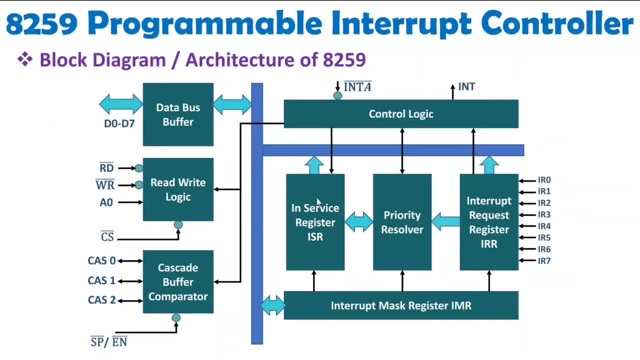 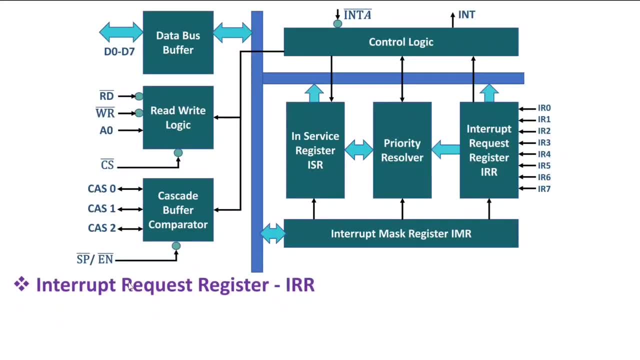 of all, I'll be going to explain you each of these blocks in detail so that you can understand working. So first of all I'll explain you all the blocks step by step. So first of all I'll be explaining you. interrupt request register IIR. You can see it is available. 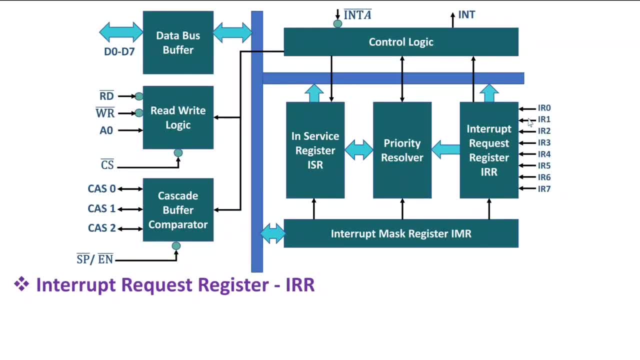 over here. It can take eight different input interrupts, IR0 to IR7. And based on whatever interrupts comes over here, bit of that register will get set to one. For example, if I say IR0, IR1 and IR2, that is generated simultaneously, So IRR register status will be having these. 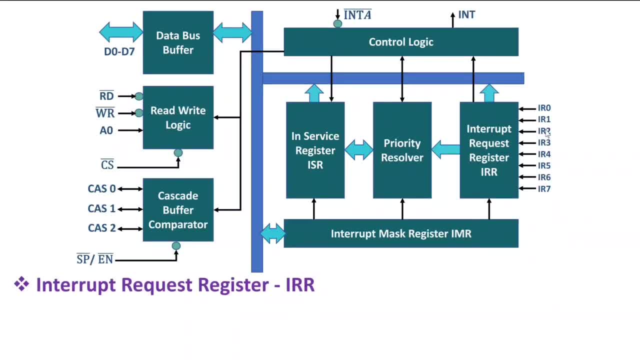 three bits: D0, D1 and D2.. These bits will get set to one Right. So here we have total eight interrupts, IR7 to IR0, with IIR register, And here it is eight bits register Each. 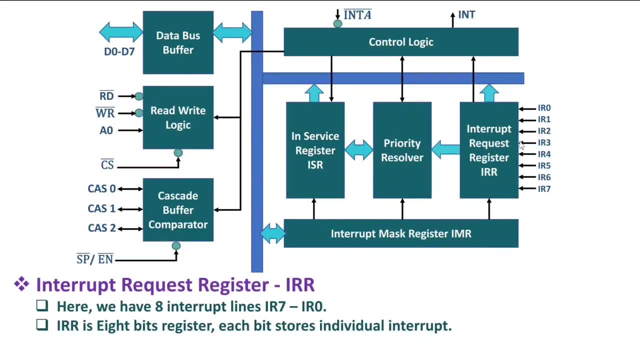 bit stores individual interrupts. If interrupts are generated simultaneously, then IR1 and IR2 are generated simultaneously is generated here, that bit will get set to 1, and when interrupt occurs, that corresponding bit gets set to 1. and now that data will be given to priority resolver. right now let us see next block. 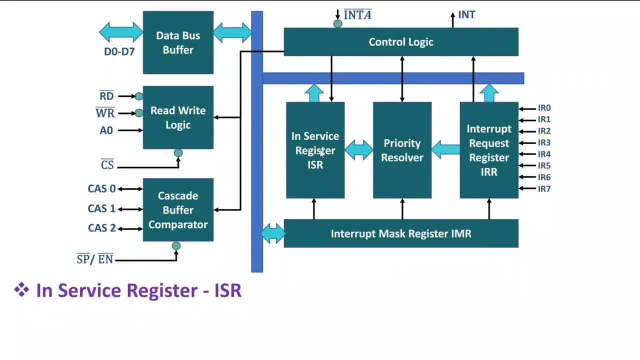 that is in service resistor, that is this block over here. my dear students, this in service resistor block gives you idea about which interrupt is there in service. so it is also of 8 bits. let us say right now this: 8259 is connected as per fifth interrupt request in service, like ir5 that is. 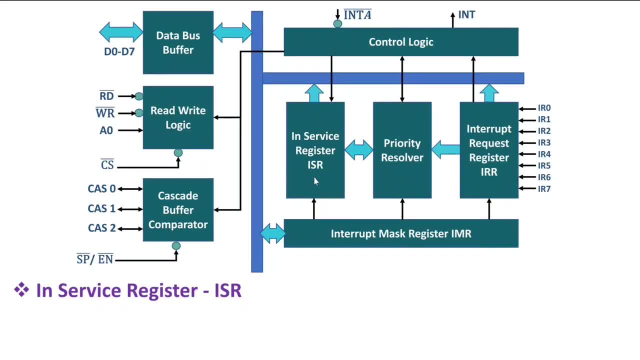 there in service right now. so what will happen? as ir5 is there in service right now, ir5 bit will be 1 and that indicates what it indicates: 5. 5th interrupt terminal is there in service right now. right, so this is of 8 bits and it shows you. 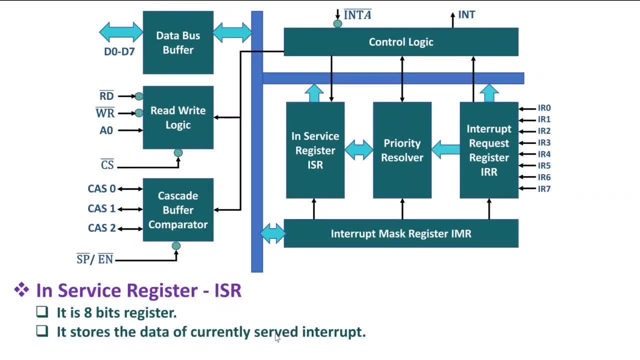 status of which interrupt is been served right now. now, my dear students, let us try to understand next block, that is, interrupt mask resistor. so this resistor is also of 8 bits and it is showing you status which interrupts are masked right now. right, so whatever interrupt is masked, 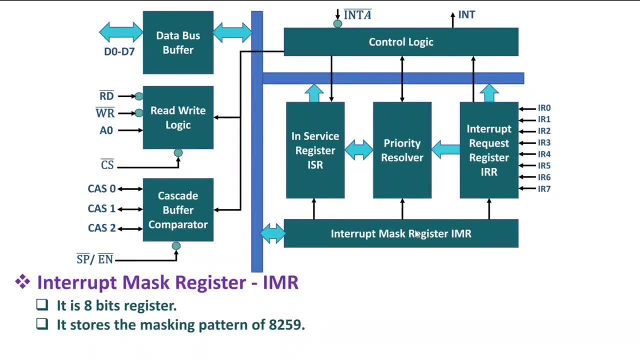 then 그래요 here, correct process which I had showed you right now over here. on that, you will be providing logic 1 bit right, so it will be having B 0, 2, D, 7, for example, if you want to mask, I are 3. 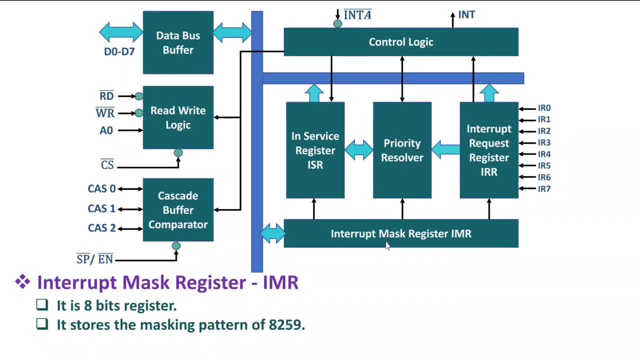 and I are 4, so d 3 and d 4 bit of this resistor should be 1. that indicates that resistors are masked right now. so individual bits will hold masking of individual inter up over here by. I am resistor right now. my dear students, I'll explain you: priority resolver, so see. 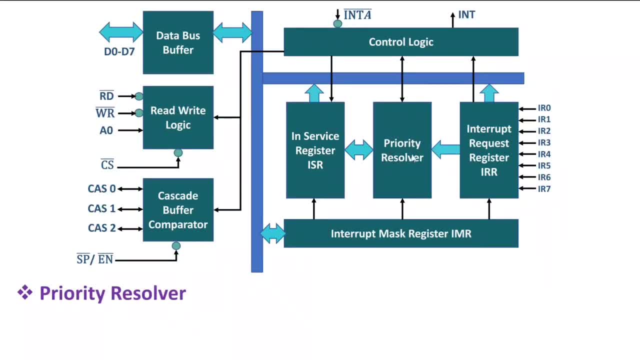 priority resolver that will be taking information from interrupt mask resistor, from ISR resistor as well as from IRR resistor, and by taking information from this three block it will be deciding highest priority of interrupt and, based on highest priority service to the interrupt will be given all right. so it 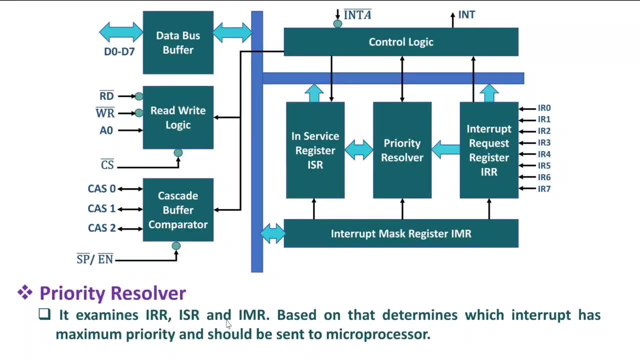 examines IRR, ISR, IMR and based on that, it will determine which interrupt has maximum priority and should be sent to microprocessor. after that, let us see what is happening with logic control. so here, my dear students, with control logic, we have two terminals: int and int a bar. this int is connected with int, our. 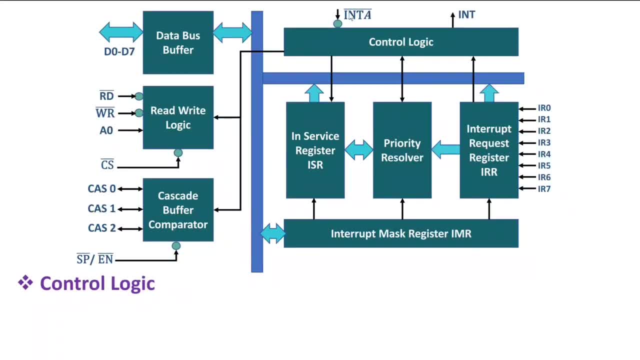 terminology: microprocessor 8085 and this int, a bar terminal that is connected with int, a bar terminal of microprocessor 8085. so once you decide that which interrupt should be served right now, intr signal will be given to 8085. that is interrupt request and based on that interrupt. 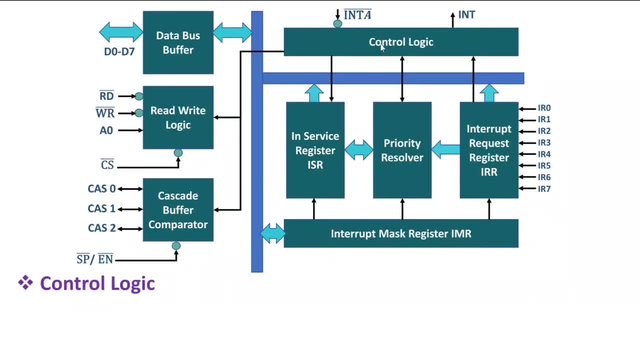 acknowledgement will be given by microprocessor to this control logic right. so here int pin is connected with intr of microprocessor, that is to send interrupt request, and int- a bar pin, is connected with int- a bar of microprocessor that is to receive acknowledgement and remaining blocks. 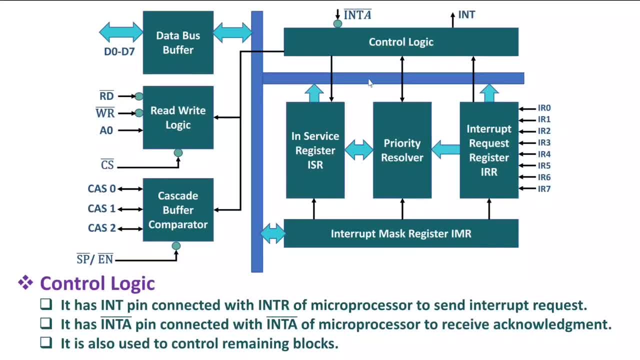 are also controlled by this control logic block. right, so this control logic block will provide controlling to remaining block also. you see, connection is been also given over here. right now, my dear students, let us try to understand what is data bus buffer. so obviously it is connected with system bus of microprocessor. 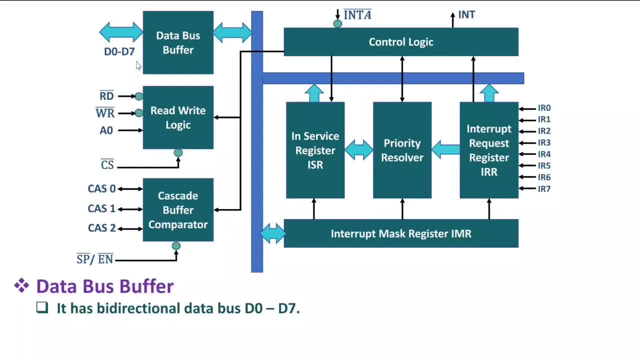 right bi-directional data bus d 0 to d 7. that is there. if you want to install control status over here, in that case this buses are used and here we can read even at the side of microprocessor: so these are been interfaced with the microprocessor system bus. 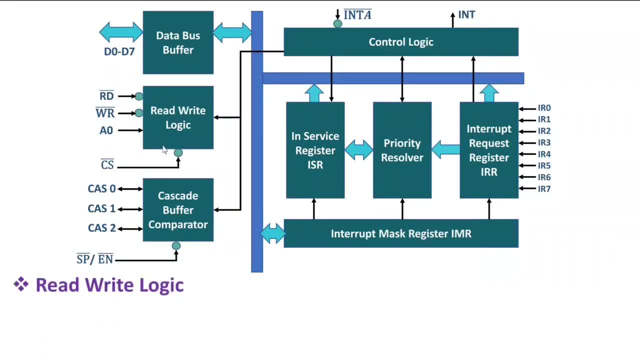 right now, my dear students, let us see what is happening with read, write logic. so read bar and write bar that is connected with microprocessor to read and write data and chip select that we connect to have a selection of chip, which is this chip of 8259, right, and here this block is also. 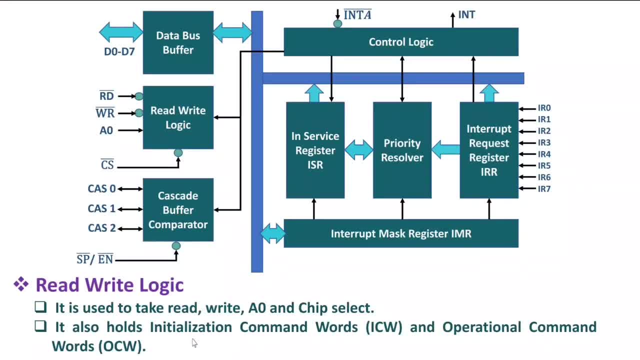 holds initialization command word. this is very essential whenever you initialize this 8259, at that time initialization command words that should be given and there are various modes, which is there with 8259 for that operational command word that should be given to it, right? so that is. 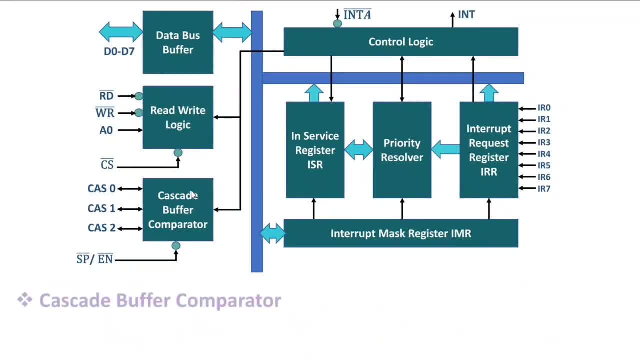 been there with this. read, write logic. now, my dear students, let us try to understand cascade buffer comparator. here, as i have said, with 8259 we can have multiple 8259 connection and for that we need to have one master 8259 and eight slave 8259 that can be interfaced by this cas0, cas1 and 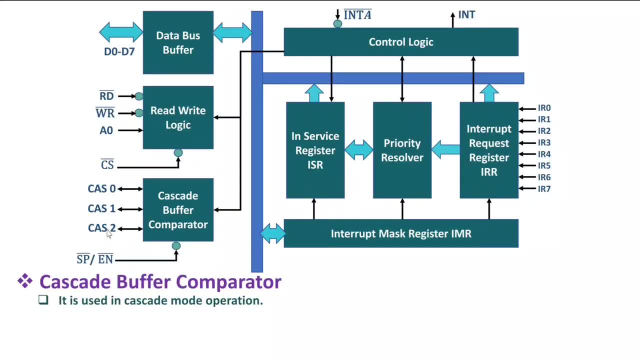 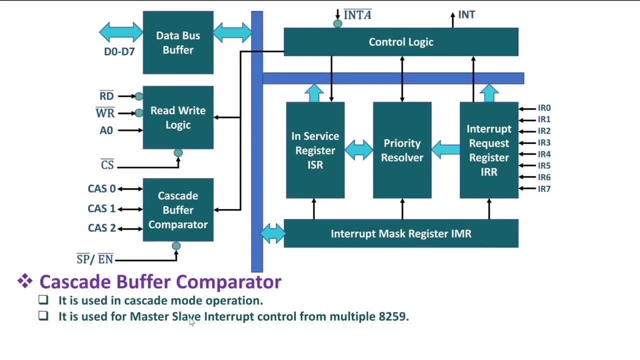 to 64 interrupts where we have master slave configuration. right here this terminal sp bar en bar. that is to enable that master and slave. so sp en bar. that gives you idea about slave program master enable line in buffer mode. you will be observing it is functioning as enable line. 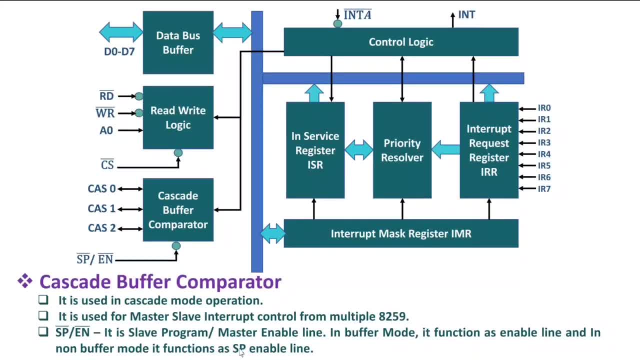 And in non-buffer mode it functions as SP enable line, right. So that is how this block is there. Now, my dear students, I'll explain you how this 8259 IC is working. So, first of all, INTR of 8085 must be enabled with EI instruction. 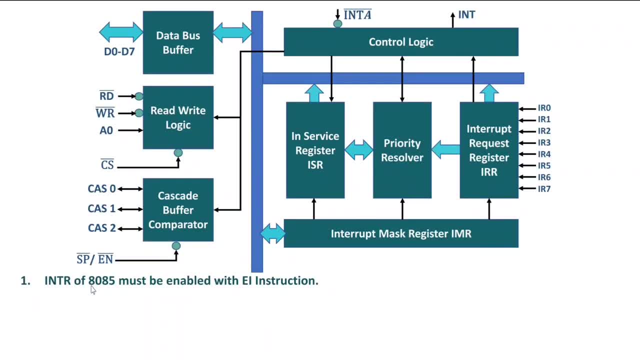 My dear students, if this INTR line is not enabled, then 8085 cannot take interrupt. So inside 8085, we should execute EI instruction, enable interrupt instruction. After that only INTR can take interrupt with 8085, right. 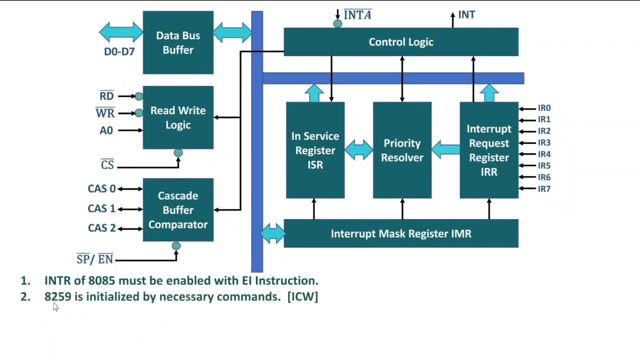 So this should be clear to you. After that, we should know that 8259 initialization that should be done By ICW command right? This is very necessary. You should know that initialization should be getting done. After that, only 8259 can function right. 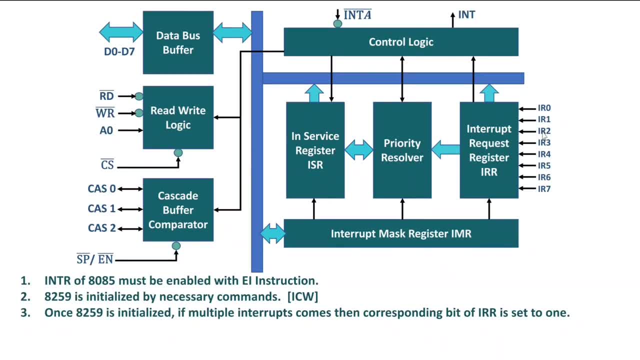 Once initialization is been done. here you see, with 8259, we have total 8 possible interrupt: IR 0 to IR 7, right, And if multiple interrupts are coming at a time, then what will happen With this resistor, whatever interrupts are coming? 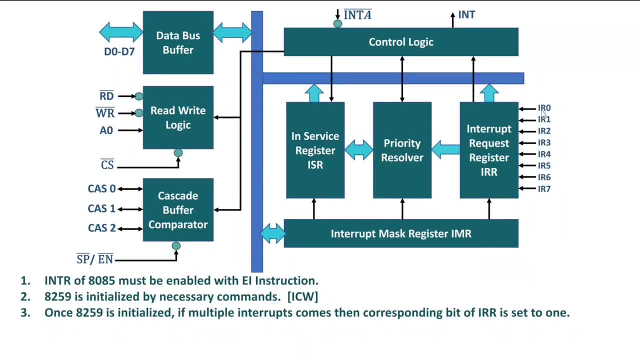 those bits will get set to 1.. For example, if I say IR 0, IR 1 and IR 2, these three interrupts are set to 1.. So D0, D1 and D2, those three bits that will get set to 1 over here. 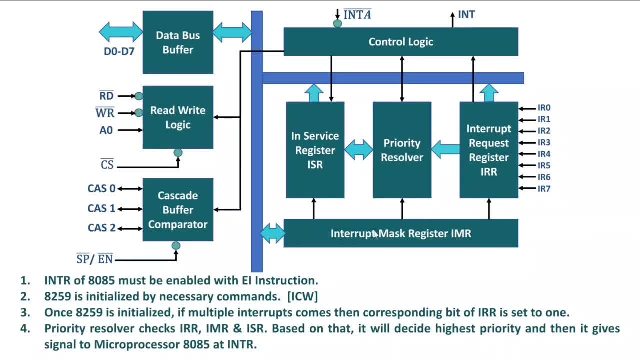 After that, priority resolver will check the status of IIR, ISR and interrupt mask resistor. As I have said, this ISR in-service resistor that will be holding content of which interrupt is there in service right now, And IMR that is having a data of which interrupts are masked right now. right, 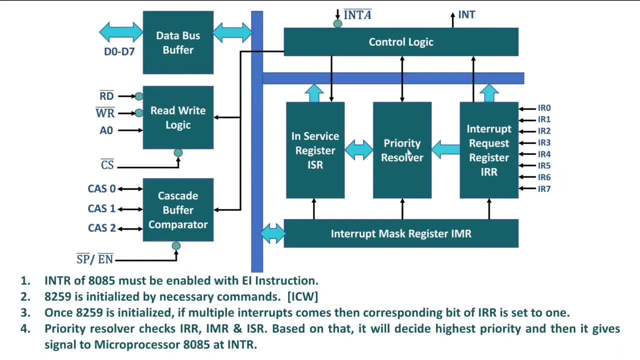 So that will get checked by priority resolver and it will decide highest priority of interrupt And then, based on that, highest priority command will be given to 8085 at INTR, For example. let us say right now there is no interrupts there in service and out of this three interrupts 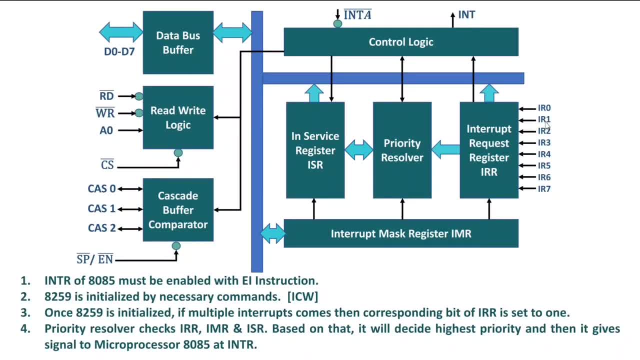 Let us say the third interrupt of INTR. there is no interrupt out there. Let us say that there is no interrupt out there in service IR1 that is having highest priority. so IR1 that will be given to the service by having a command at INT line which is connected at INTR of 8085, right, so now this IR1 will be. 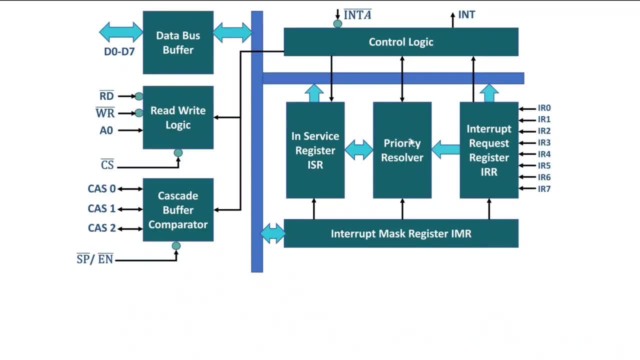 there in service right. once microprocessor receives that, it will be giving INTA bar interrupt acknowledgement to 8259 and at that time microprocessor will complete current instruction and then acknowledgement will be given to 8259 right once acknowledgement comes at 8259- my this 8259- that will be providing opcode of call to 8085. my dear students, once microprocessor 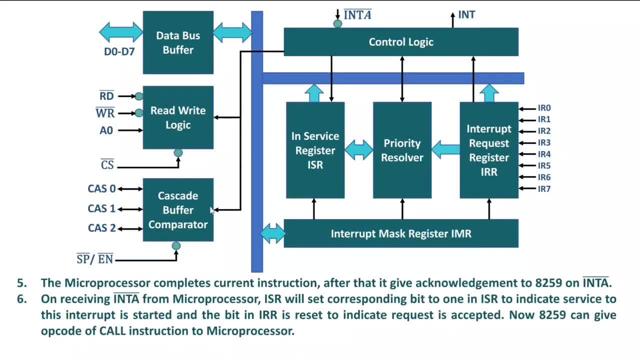 sends that interrupt acknowledgement, then you, this 8259, that will have to provide call instructions opcode, right? so on d0 to d7, call instructions opcode will be forwarded. but along with that, what is happening, you see? ISR bit will get set to 1. so here, as I have said, IR1 that is having highest priority. so 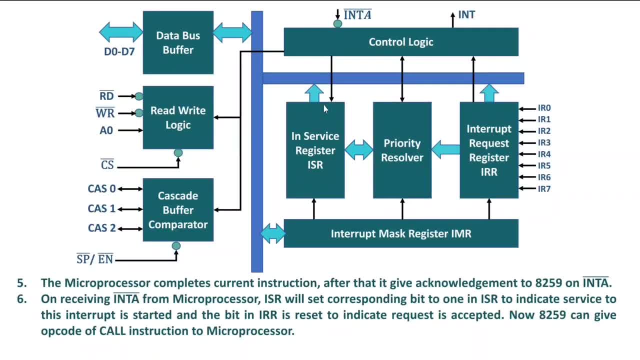 ISR d1 bit. that will get set to 1. once it is getting set to 1, it will reset the bit of IIR1 resistor. so ir, our resistor, is having ir1 which is there at d1. that will. that will get reset now. once this bit is getting set to one, this bit will get set. reset now with ir and after that. 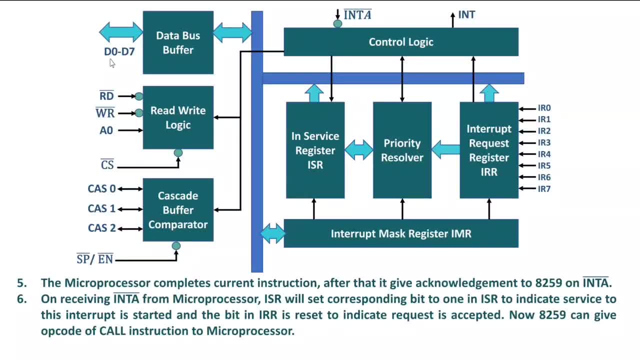 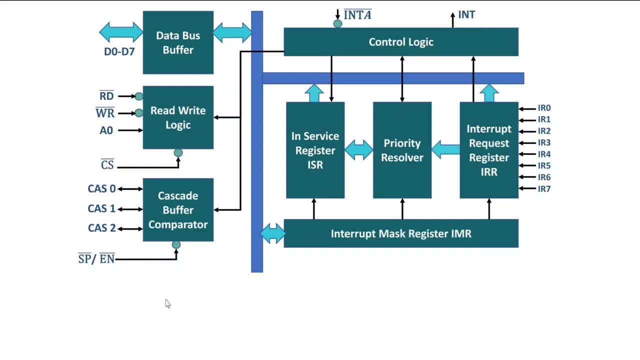 that opcode of call will be forwarded over d0 to d7 line. now, my dear students, once that opcode is forwarded to microprocessor, microprocessor will sends two more int a bar signal to 8259, and during this two signals of int a bar, 8259 will sends address. right, so you should know my. 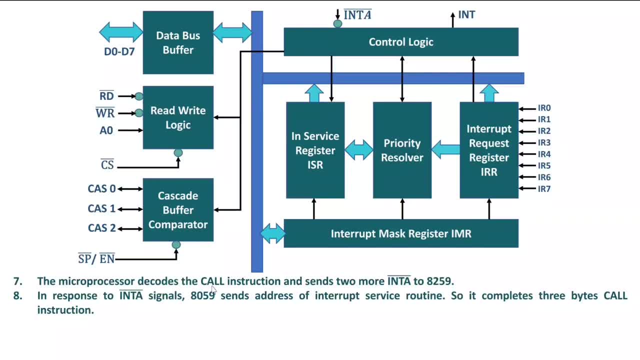 dear students, call. instruction is three byte instruction. first byte is there with opcode and next two bytes that is there with address. so those two bytes which are there regarding address at which isr should get performed, that will be forwarded in. next to int, a bar signal which is 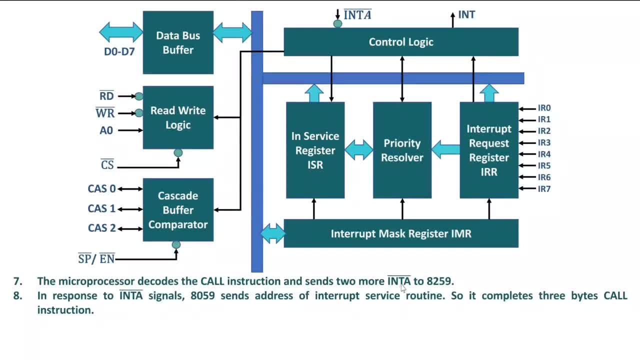 been given by microprocessor right. so in respond to this, 8259 will send address of interrupt service routine and that completes three bytes of call instruction right. and once microprocessor receives all those data which is there regarding call instruction opcode and address, it will start with that interrupt service routine by pushing the content of program counter on stack.